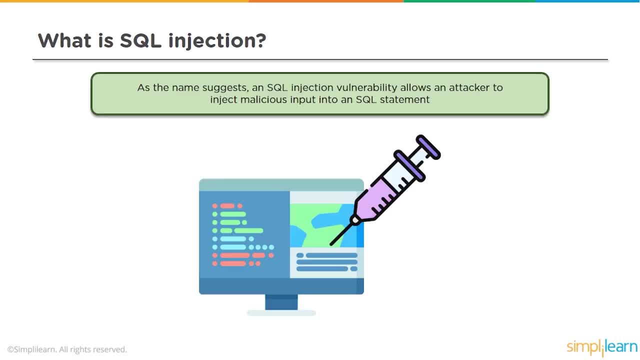 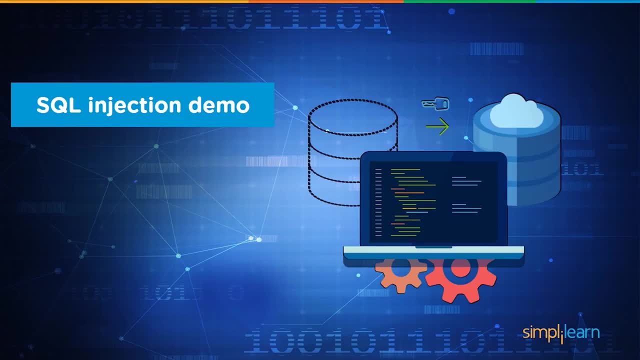 coming in, So this character needs to be filtered at the application level itself. Now let's look at a quick demo. So what we have done here is I have this virtual machine called broken web applications virtual machine, version 1.2.. I'm going to power this on. 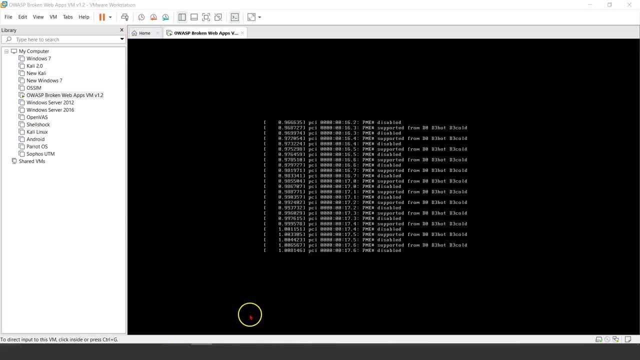 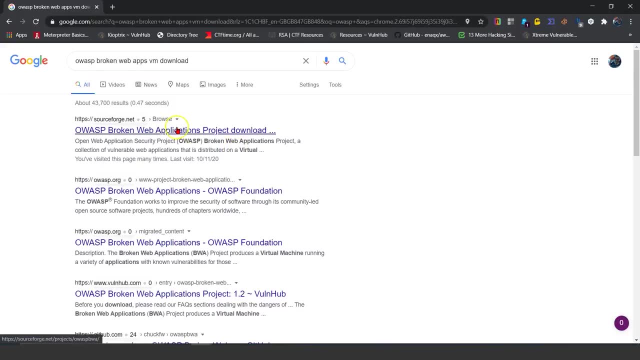 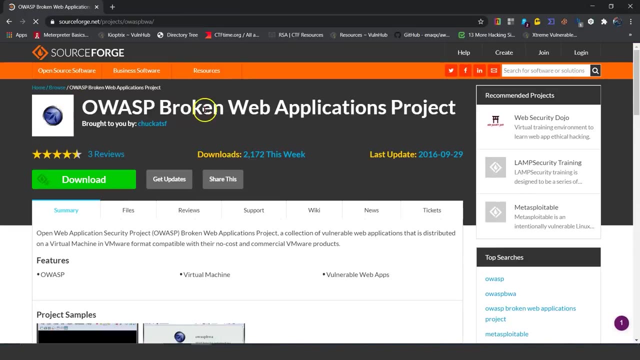 Till this power is on. I'm going to show you where we can download this utility from, So you can just look for OWASP broken web application project download. You'll find it on sourceforcenet. Click on the link. You can download the broken web application project. 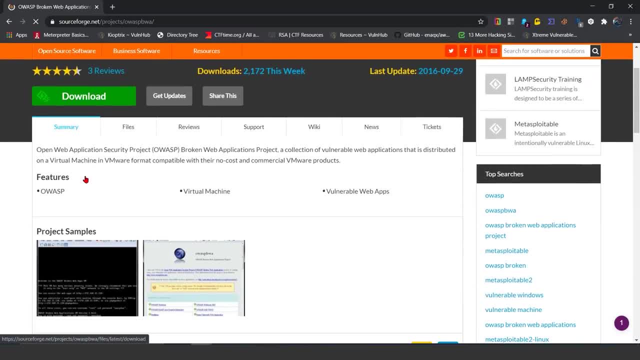 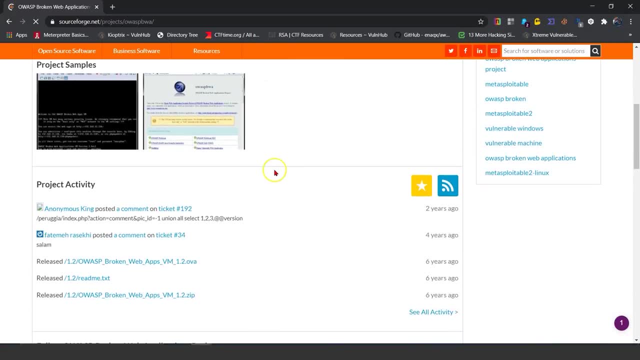 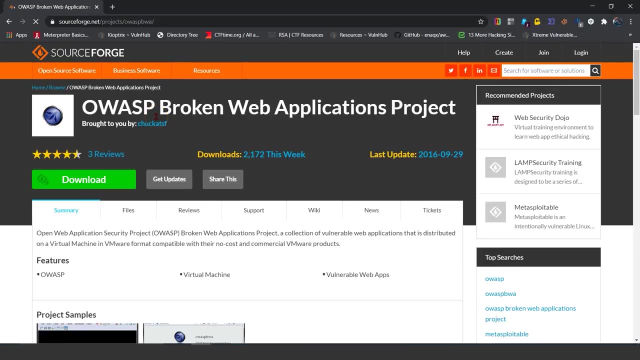 from here. This is the one 0.9 GB download and you can have a zip machine directly for VMware or Oracle Virtualbox. Now, this is an application that has been developed by OWASP, which stands for open web application security project, which is a not-for-profit organization, and periodically 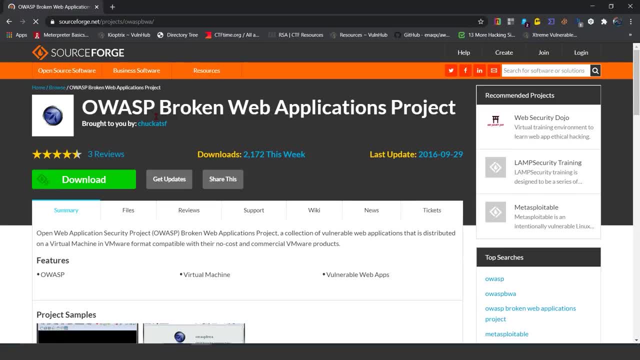 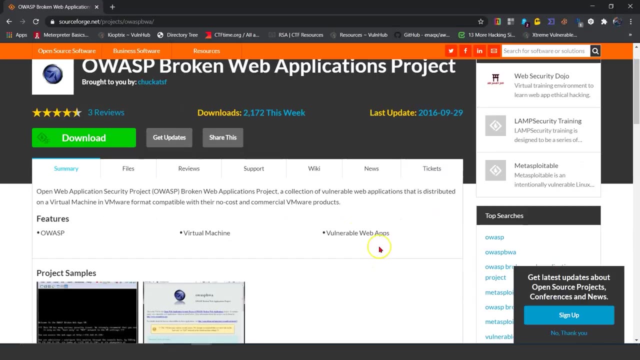 releases the most top 10 risks that an application will face for that particular year. So they have given a web application- uh, with inbuilt vulnerabilities- for professionals like us to practice upon, to develop our skills upon, because doing this in the real world is illegal. i cannot go onto a website to demonstrate. 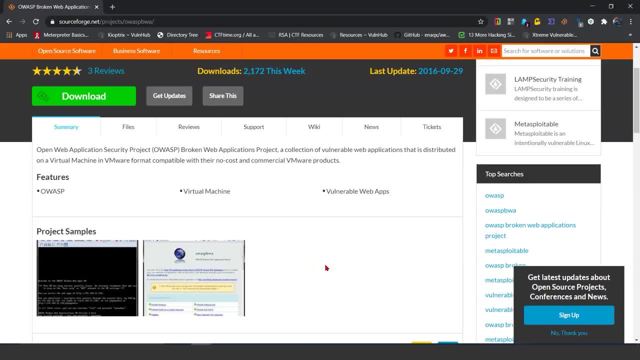 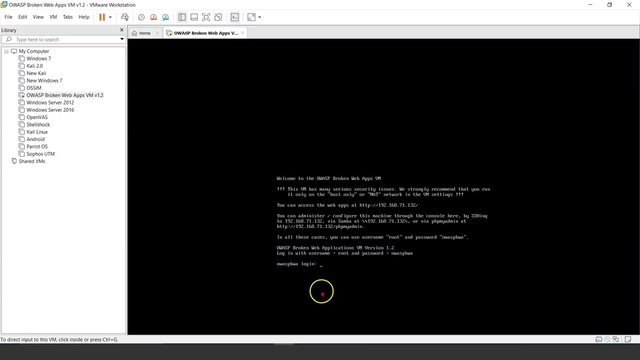 how a sequel injection attack works. uh, neither should you try your hands on it till you become very well rehearsed with it. so till to upgrade your skills, to upskill yourself, please download this machine hosted in a vmware workstation or an oracle virtual box, and you can then try your. 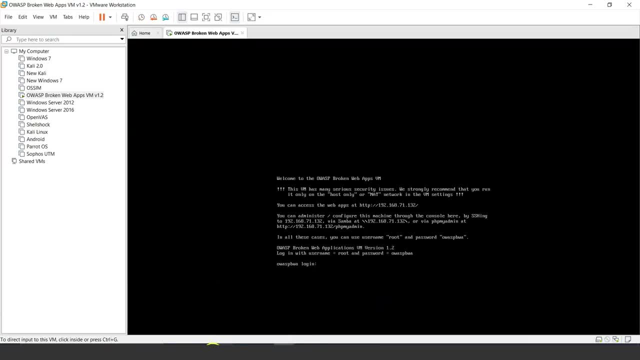 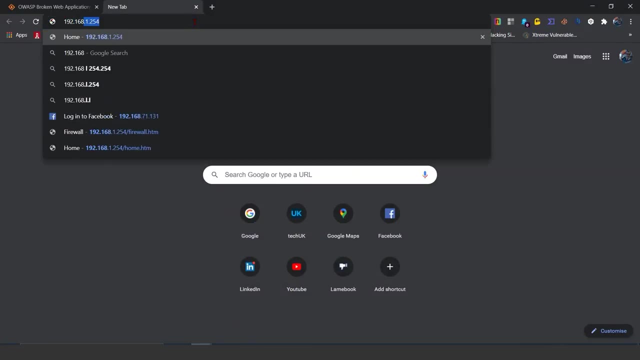 skills on it, right? so just going back to the browser here, if i open up a new tab, you will see that this machine has booted up and has an ip address called 71.132. so if i just go onto that ip address and i type in 192.168, 71.132 and you'll see the oasp broken web. 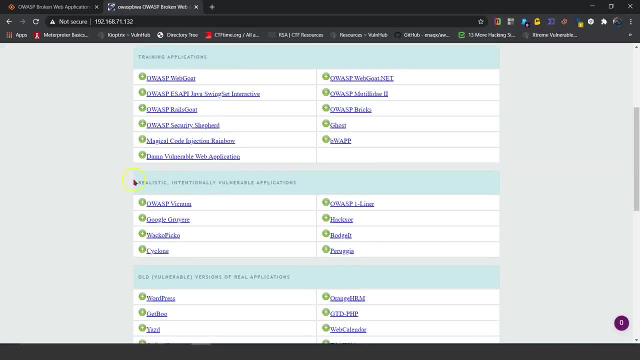 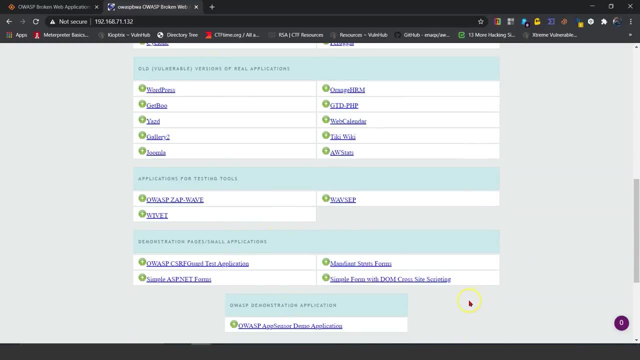 address and you'll see the oasp broken web address and you'll see the oasp broken web application project and there are a lot of training applications, realistic, intentionally vulnerable applications, old versions of real applications and so on, so forth. so there is a lot of applications inbuilt over here that you can try your skills upon. we are going to try to use. 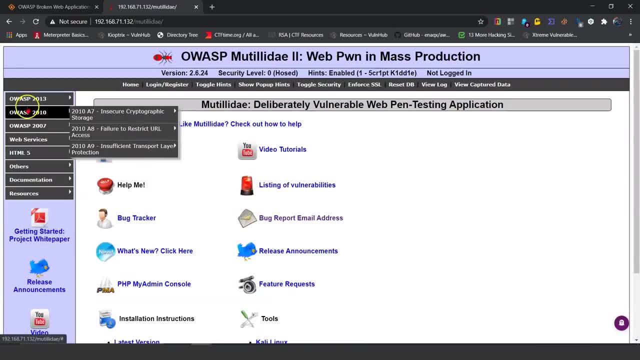 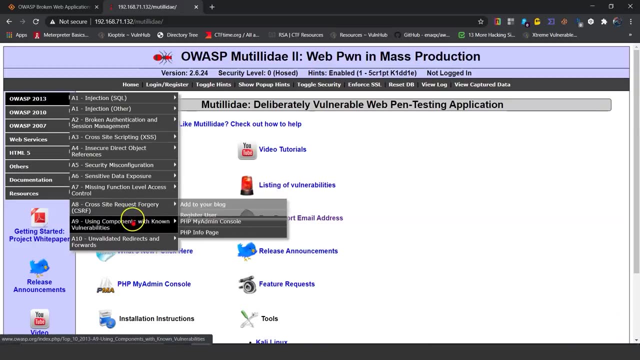 the oasp utility over here. uh, this gives you the oasp top 10 risks for 2010, 2013, 2017. is the that some of these have changed, but not all of them? uh, the order has changed a little bit, but you can see that sql injection is on the top a1 amongst the injection attacks. right, and you can. 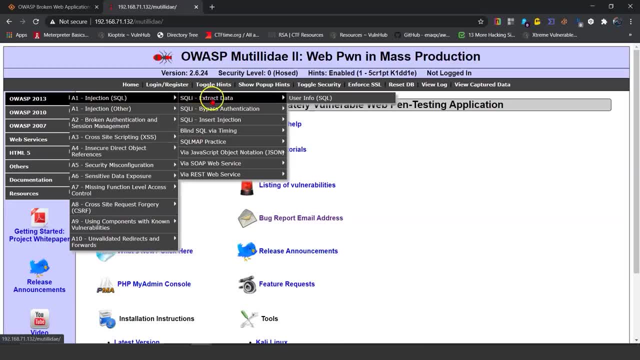 see there are multiple types that have been given here: the sql injection for extracting data, or sql injection for bypass authentication or insert your injection. uh attacks blind sql injection. and then there is a tool called sql map which is available freely on your linux machines- kali line linux or parrot linux, whichever you want to use uh for your practice targets, and so on, so forth. so 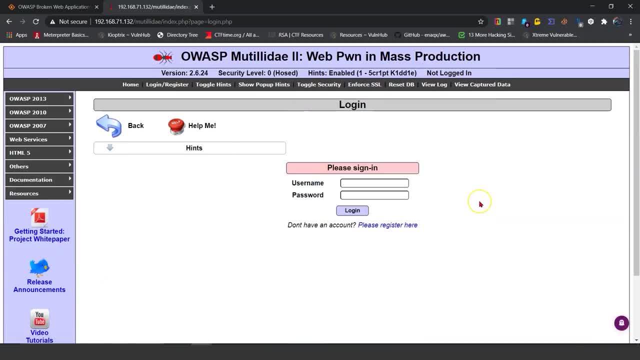 if i just take you here for bypass authentication- and this is a regular login page that an application may have, right, you look at a username, you look at password, you type that in and you log in. so let's say i don't know a password here, i'm just going to type in the username, test password. 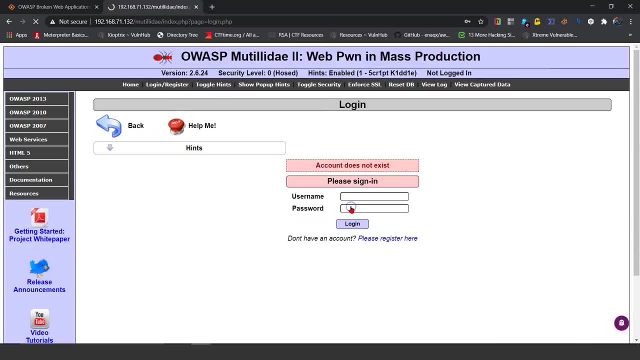 is p-a-s-s-w-r-d. i'll try to log in and it shows me that the account does not exist. the authentication mechanism does work. i did try type in a username and password. it wasn't recognized, so the account does not exist. now let's try to type in a sql query here. i'm going to just 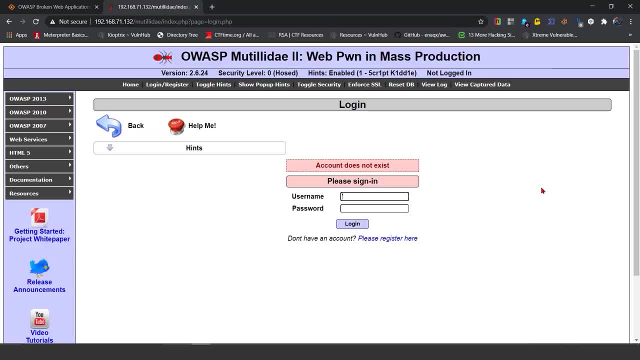 give it a single quote, which is an operator that is recognized by the sql language which, when the database tries to execute uh, will cause the database to dump some data or to bypass authentication, in this case, and i'm going to give it a condition: single quote or one equals one space, hyphen, hyphen, space, and i'm going to click on login now, right. 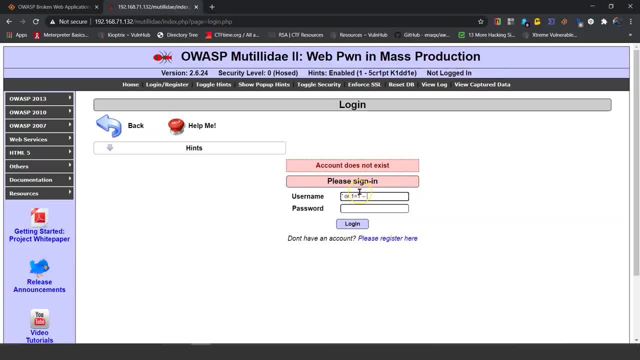 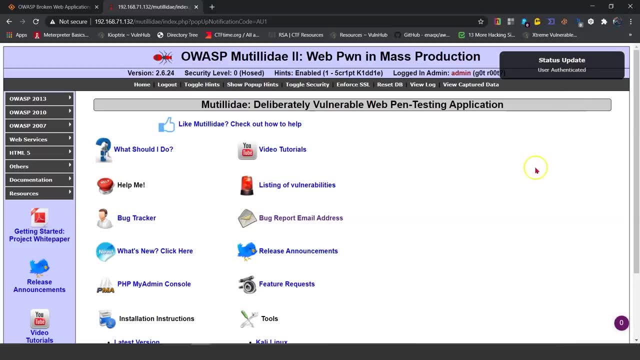 now i'm not logged in at all and we tried our username and password and we weren't able to log in. so now if i log in, you will see that it give me a status update saying the user has been authenticated and i'm logged in as admin got root. so that is what these sql queries can achieve. 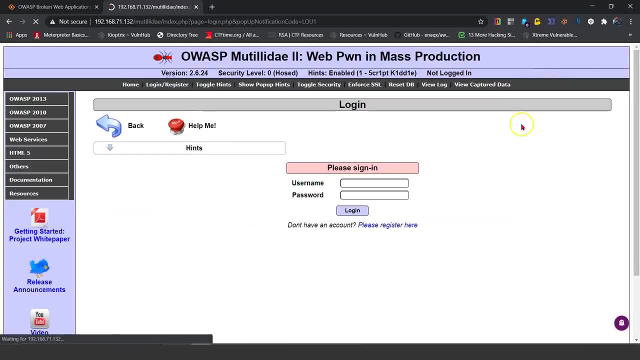 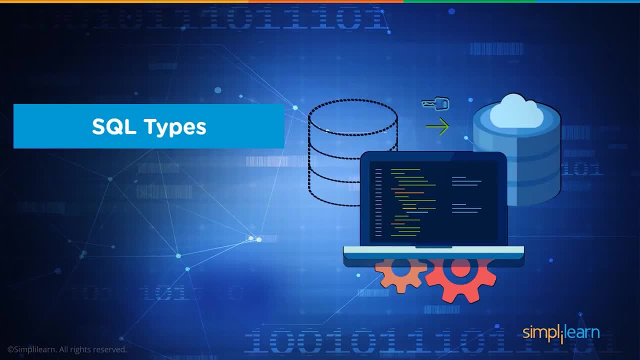 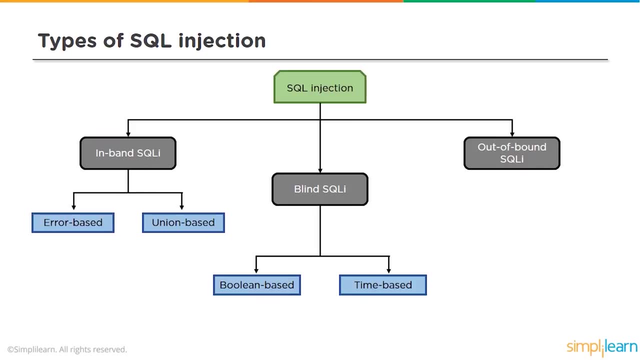 i'm going to log out right now and we are going to look at the basics of sql injection. so, looking at that small demo, looking now, let's look at what types of sql injections are available. so the first is in band sql injection, the. there are two subtypes within: in band error based injection attack and a union based injection. 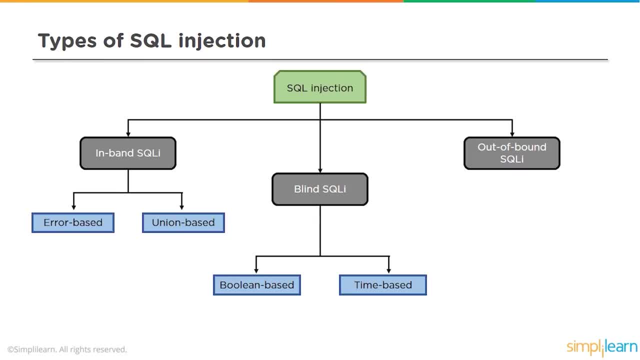 attack. the second type is blind sql injection attack, where there's a boolean based and a time based attack, and the third one is out of bound sql injection attack. now, what is in band? sql injection attack in band is where we are either attempting the error based or the union based. what is error? 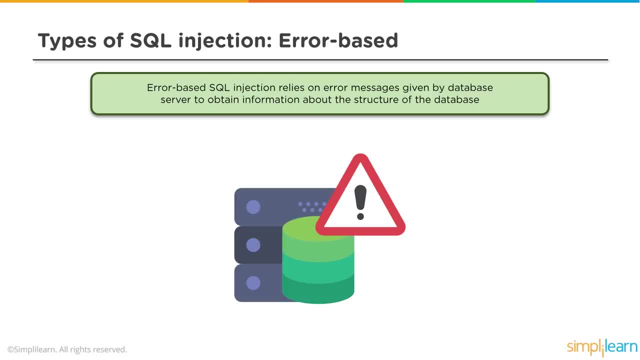 based uh. we send a query to the database, we craft a query to the database and uh, it generates an error miss message and it dumps the error message right in front of us on the screen. that makes us realize that there is a flaw and there there is some information. 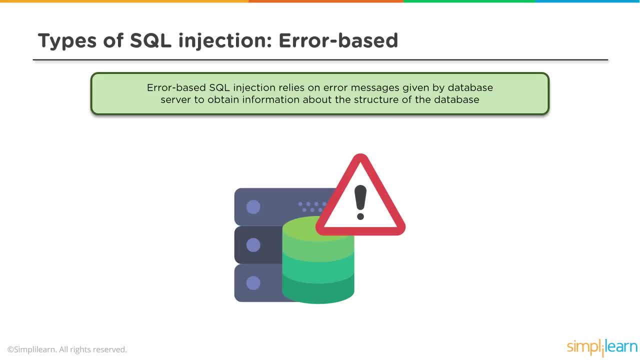 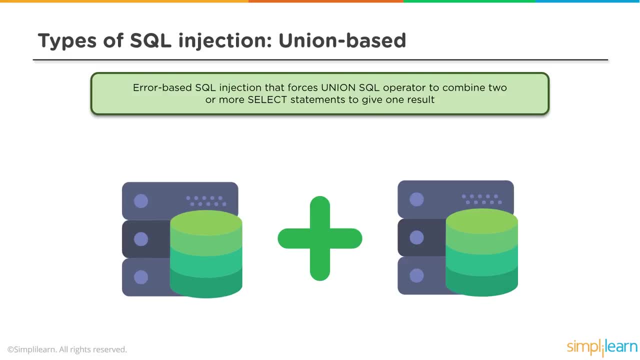 that is dumped on the screen, which we can then further utilize to craft our further queries as we go forward, go ahead. whereas union base is the, it is where we combine multiple statements at the same time. so if you look at the url earlier in the url, you would see a large structure in that url. we can 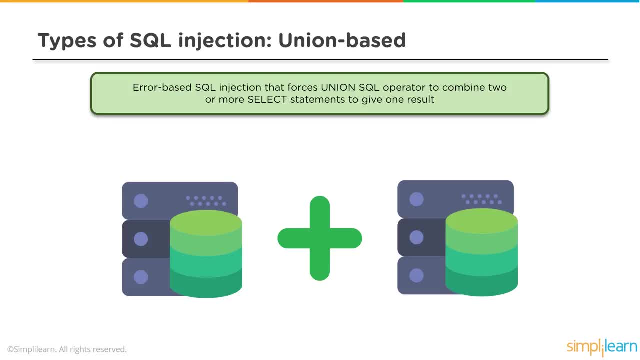 try to add more, two or more statements within the url itself, to combine them and then confuse the database into executing both the statements together and giving a data dump at the same time, right? so what would a error based uh sql injection look like? if i go back to the same database, uh, which is here, right? and if 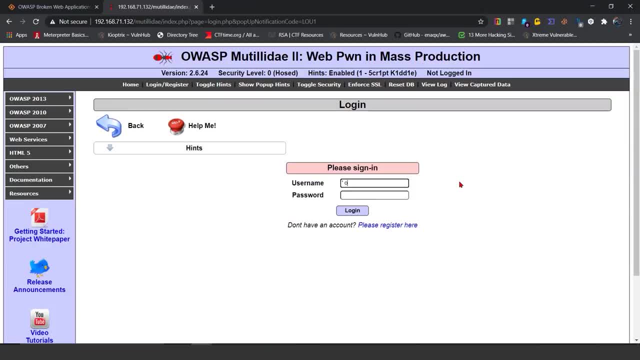 you remember the username. we gave it a single quote, or one equals one space, hyphen, hyphen, space. we gave it the condition right. so basically what it did was this: a single code is an operator that goes to the database. selects the default uh table in the user tables in this database column. 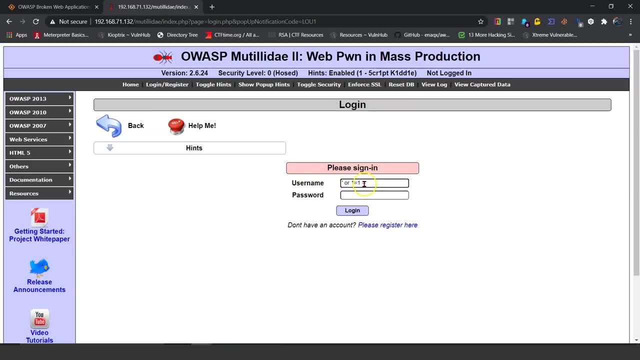 and then compares it to the condition that is given. so the condition that we gave was 1 equals 1, which is always true. so what it did was it selected the default user table that was available in the database and, instead of comparing it to a password, it compared it to the condition. so if i give it 1 equals 2, where the condition is false, 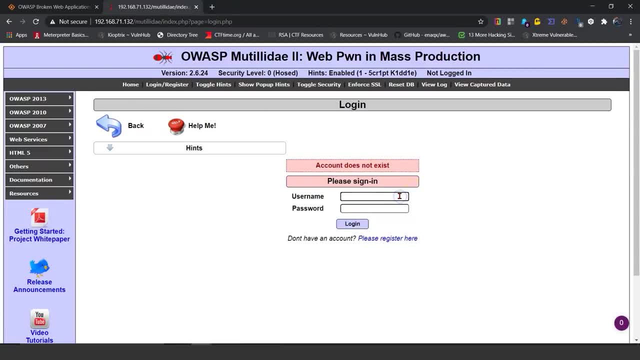 and if i log in you will see that the account doesn't exist- comes back again because the condition was false and instead of comparing the user account to the password, it basically gave the user account to the condition. so if i give it a single quote, or: 1 equals 1. 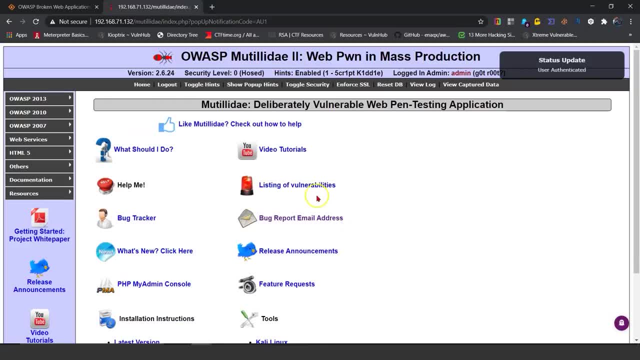 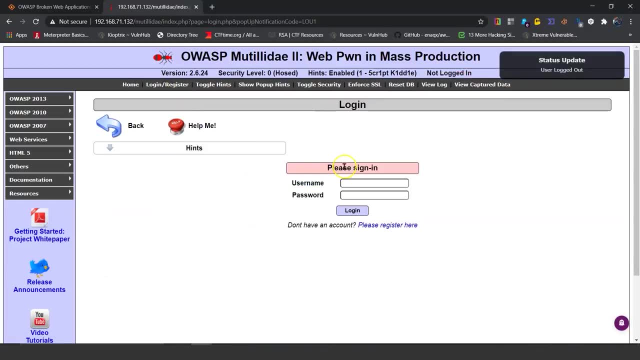 hyphen, hyphen space and log in. you can see that this is a correct condition and thus we are able to log in now. before we even go to that extent, if i just forget the condition over here and i just give it a single quote: the operator and i send this operator to the database and i click on. 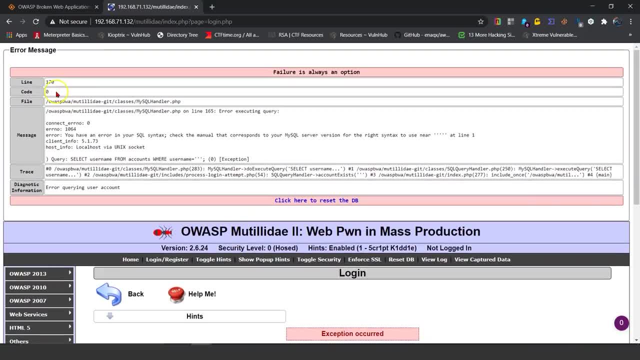 login, you will see that it generates an error, which is right on top, and it tells us the line, the file where the error happened- and you can see it happened in the mysql handlerphp file, right. and then it gives us the message: you have an error in your sql syntax. check the manual. that 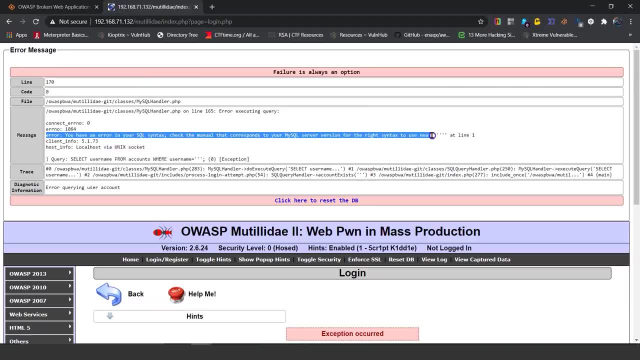 corresponds to your mysql server version for the right syntax to use. now, why would a hacker want to do this in the first place? because there are different types of databases. so there is a mysql, msql or microsoft sql, oracle, sql, ibm, db2. all of these are variations of the sql. 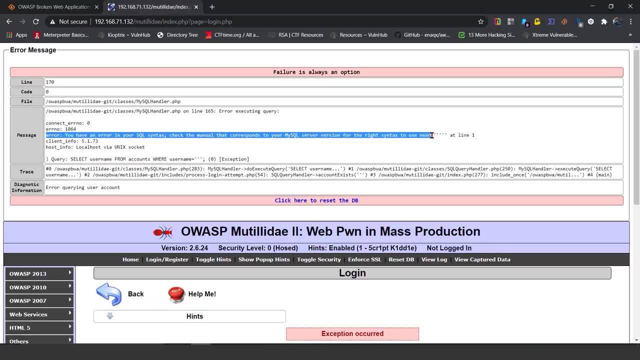 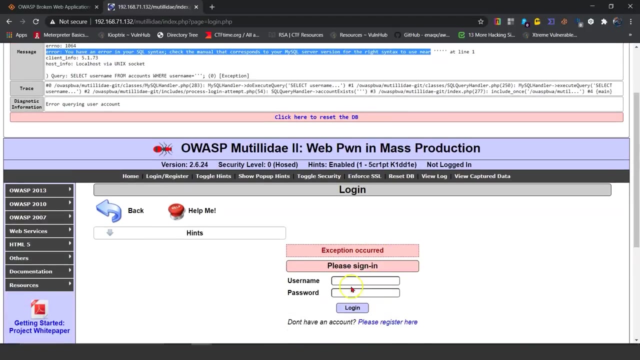 database. they use the sql language. however, every database has its own command right there, they have their own syntax, they have their own specific commands that are utilized for the database. so in this scenario, the hacker wants to identify what database is being currently utilized so they can craft those particular queries. so now with this injection, with just me sending the quote, 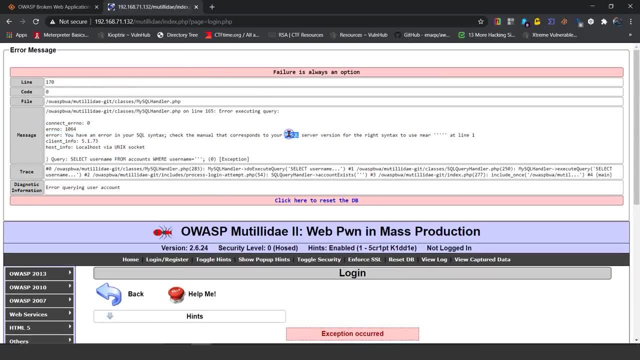 and the error getting generated. i now come to know that we are using a mysql server and the version of that server is 5.1.73, and the rest of the information about where the handlers are located and so on, so forth. right, this gives the information to the. 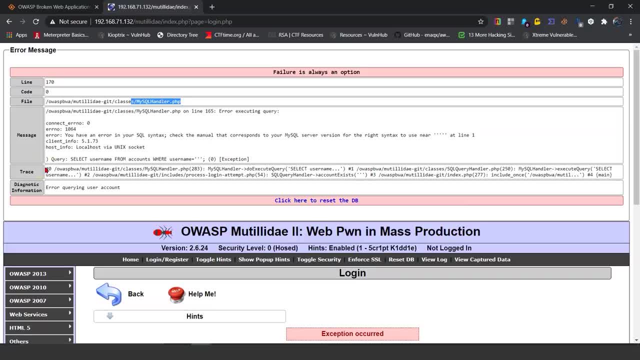 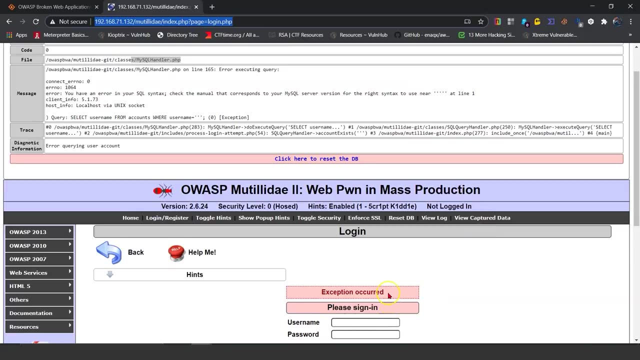 hacker of how they want to proceed next, what kind of queries they want to create, what kind of syntax they want to utilize. so error based attack is where you generate these kind of errors and you get this information. the union base is where you craft your queries within the url or you can try to combine multiple statements within the input fields. 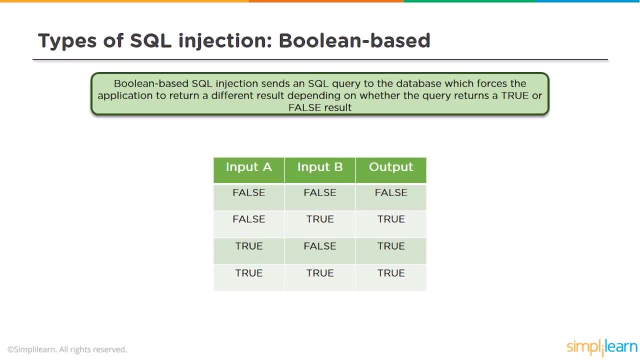 and try to generate a response from that. then we come to boolean based sql injection sends a sql query to the database which forces the application to return a different result depending on whether the query returns a true or a false result. so basically, if the input is false, the input, both the inputs- are false, the output would be false. 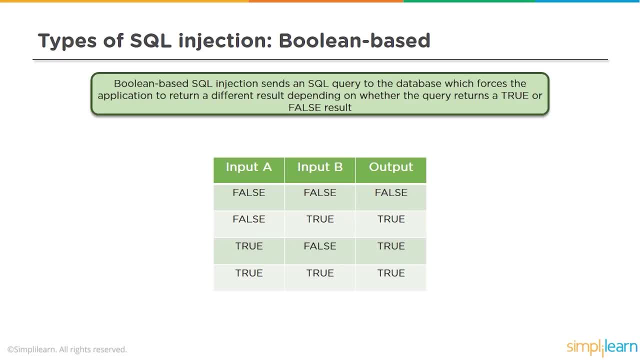 and so on, so forth. right, so depending on the result from the inputs, the attacker will come to know which input is true. with this, he can then access the database of the website. so you're trying to figure out by sending out multiple inputs and then analyzing the output to see. 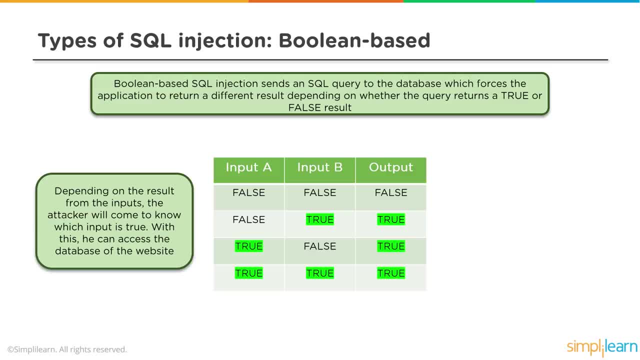 what exactly, which command exactly worked? what was the resultant output of that command? thus, from this kind of an information, the hacker can infer their next steps. so let's go to the next step. let's see how to do it. so let's go to the next step. 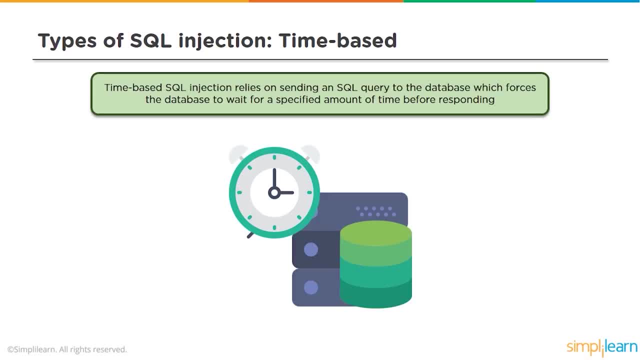 forward. Then you have time-based SQL injections. Now there are times when a database administrator or an application administrator has done some security configuration and does have disabled verbose error messages. Now, what is a verbose error message? The error message that we saw right here. 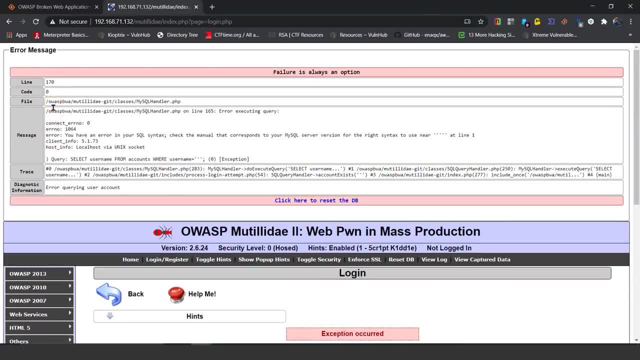 is a verbose error message. That means that the message gives out details. The message gives out details about what the database is, the version and whatnot. So if they have sanitized these errors and you no longer can generate these errors and thus you cannot figure out, 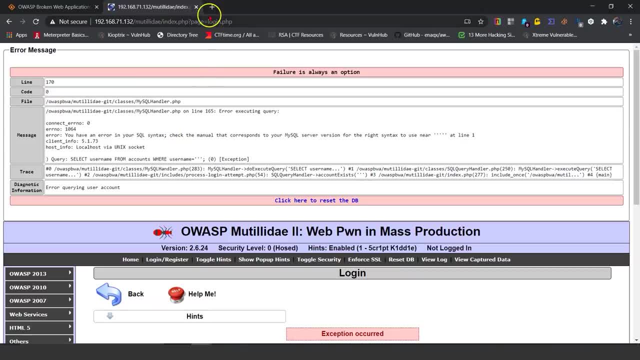 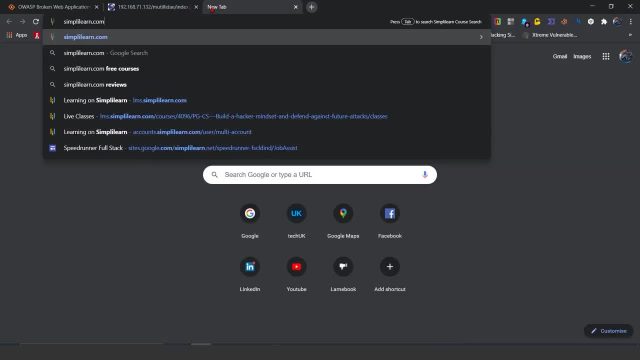 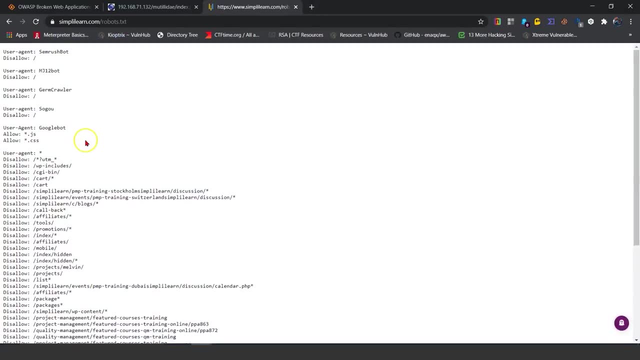 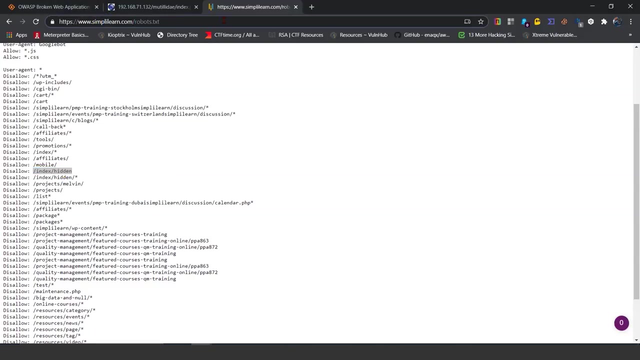 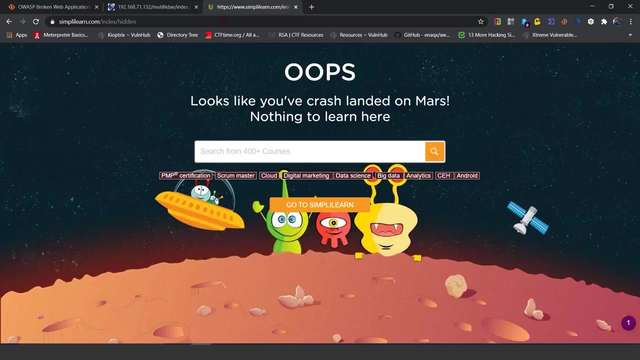 what database is then? what do you do right? For example, if I just take you to simply learn the database, I can take you to the URL that is supposedly not accessible. You can see that it gives a generic error. Oops, it looks like you have crash landed on Mars. It doesn't give you a. 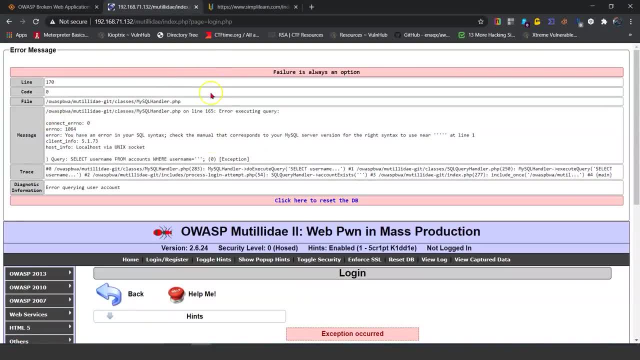 verbose error that we saw here. So this gives us a detailed error of what went wrong, where it gives us the database, the version of the database and what the database is. So if you take you to a URL that is supposedly not accessible, you can see that. 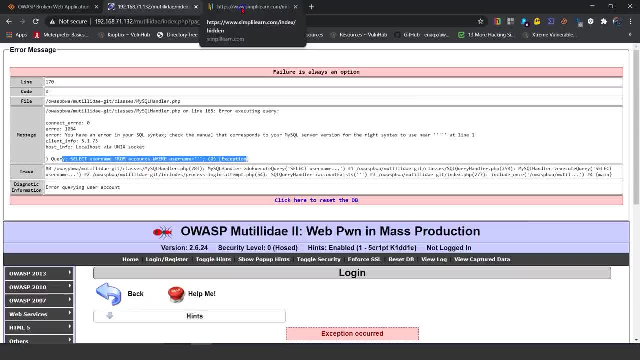 where the query went wrong and et cetera, et cetera, et cetera, Whereas on this site, where there's some, there's a lot of security that goes in here, So you can see that it doesn't generate. 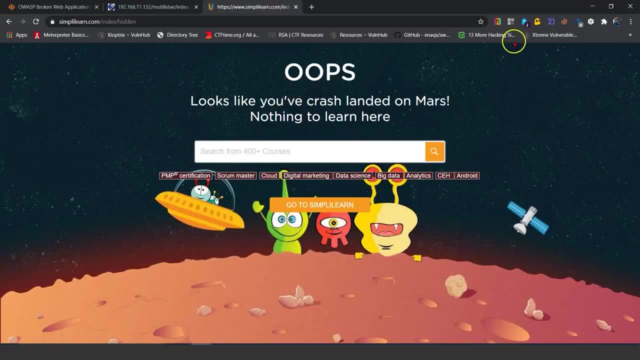 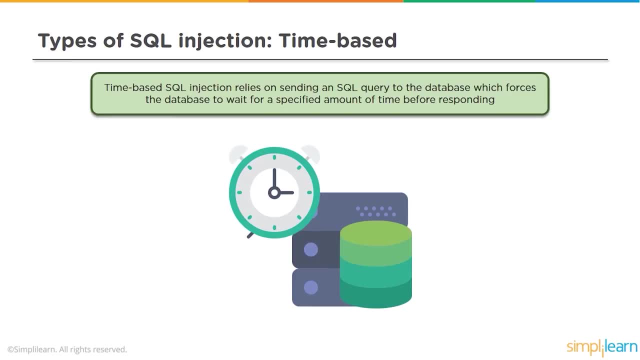 a error, It just get a generic page in front of you. So in that case, what does a hacker do? So the hacker then injects a time-based query in the URL which allows us to verify whether the command is being executed or not. So we put in a time weight. 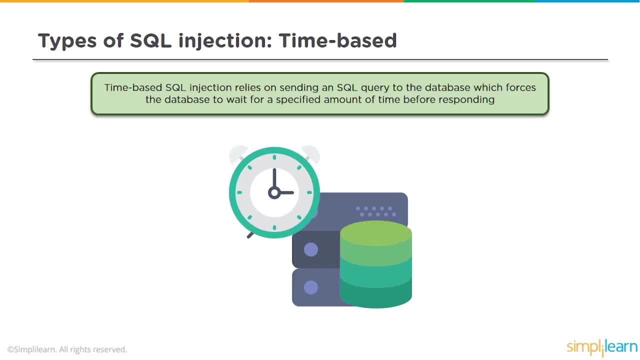 Let's say, 10 seconds of time weight. So if we, the moment we inject the query, if the query times for 10 seconds and then gets executed, that means that the SQL injection is possible. However, if we inject the query and uh, it just gets executed without the delay. that means that the time uh. 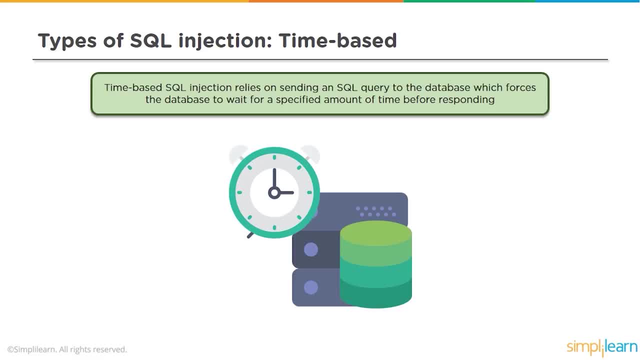 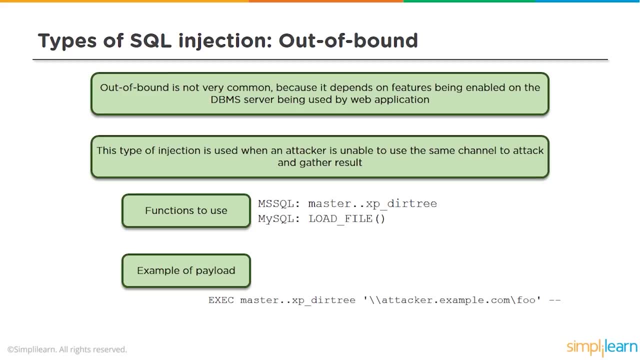 the injection attack would not be uh possible on that particular site. Out of bound is not a very common attack. It depends on the features being enabled on the database management site system that is being used by the web application. So this can be a somewhat of a misconfiguration. 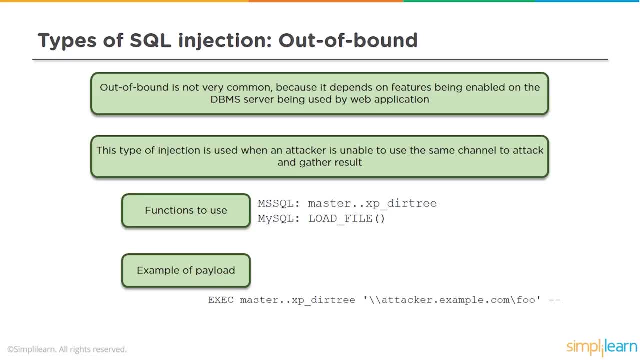 error by the database administrator, where you have enabled functions and not sanitized them. So you have not done access controls properly, you have not given account control. So queries should never be executed at an administrative level. They should always be executed at a user level, with minimum privileges that are required for that query to be executed. Now, if you're 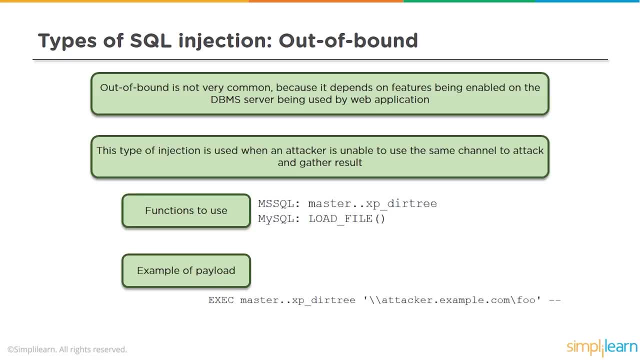 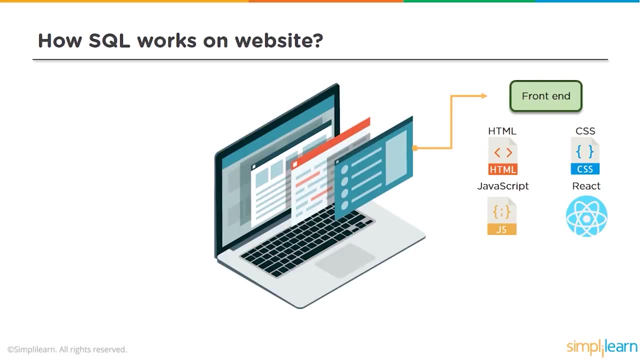 allowing these kind of functions to be enabled at the DBMS and there is an administrative account that can have access to them. at that point in time, an out-of-bound injection attack is possible. So let's look at how a website works right, How SQL works on a website. Now 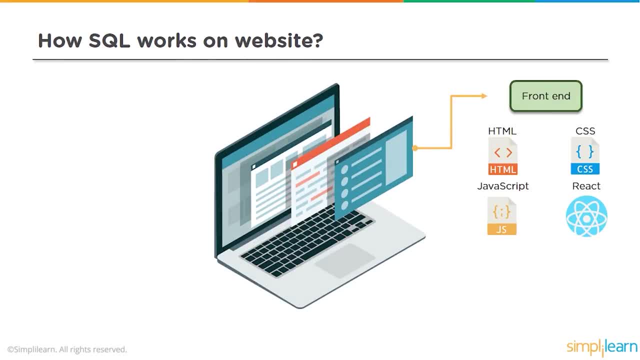 the website is constructed of HTML hypertext markup language, which would include JavaScript scripting for functionality, cascading stylesheet for the mapping of the website right, and then React JS and whatnot for the functionality. Now, when we send a query to the website, it 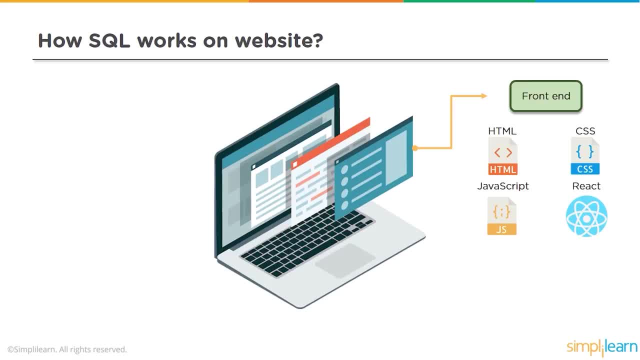 is normally using the HTTP protocol or HTTPS protocol. When the query reaches the application, the application would then go ahead and generate the SQL query. At the client side, you'll have all these scripting languages coming in on the front end that we can utilize. 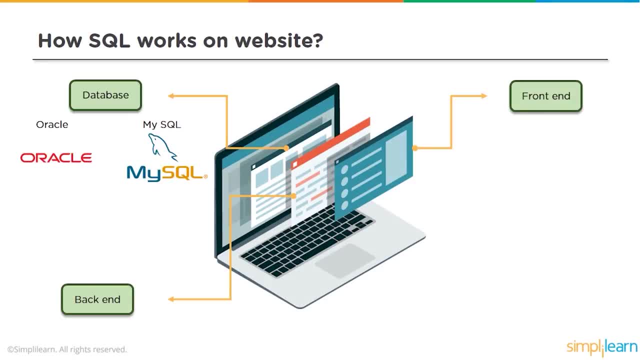 To craft queries and then send them across. At the server side you'll have databases like Oracle, MySQL, MSSQL and so on so forth that will then execute those queries right. So just to give you an example, if I use a tool called Postman- what we generally do- 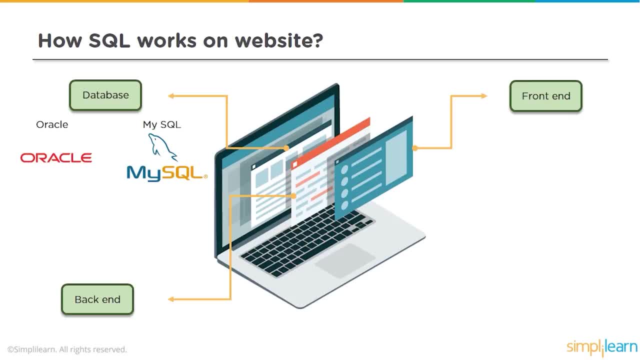 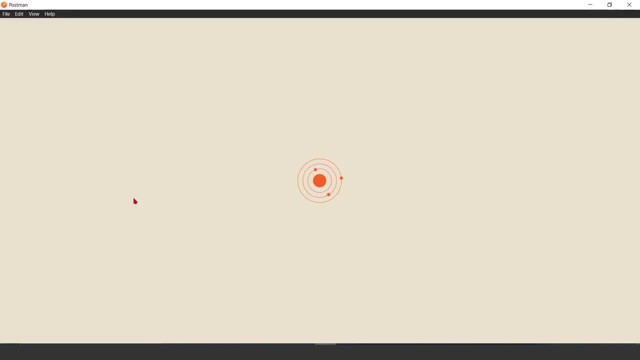 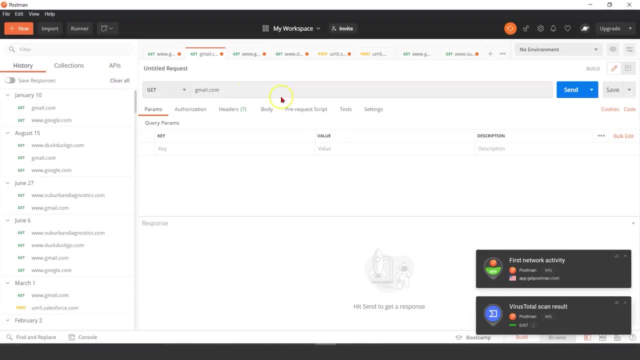 when we craft a query is we send out a GET request to the website and then we receive a response from the site With the HTML code and everything. So this is a tool that is utilized by software testers to test the responses that you're going to get from various websites. So on the left, 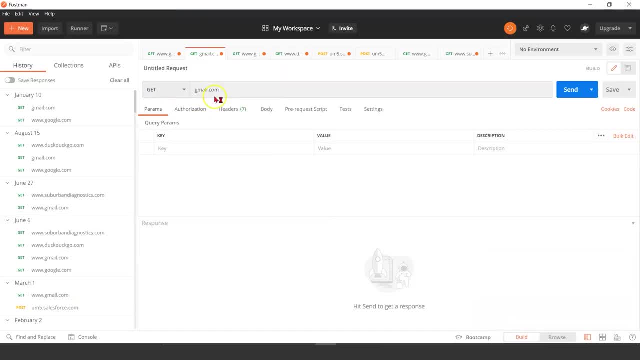 hand side. you can see I've used it on quite a bit. Here we have an example for gmailcom, So let's continue with that. So this is a GET request being sent to Gmail. The moment I send it, it's going to create an HTTP request and send it across The response that I get. 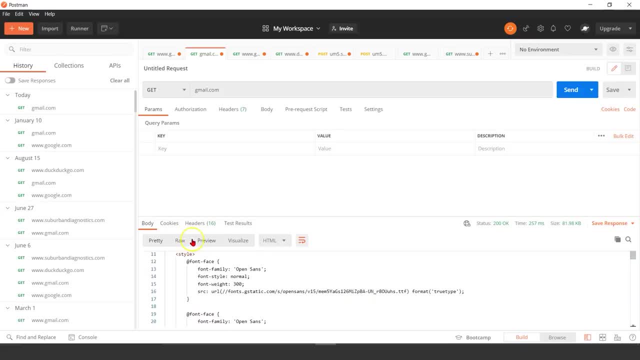 is this. This is the HTML code for gmailcom, right? So I can see that these are the codes that are being sent to the website. So this is an adress that has been sent through Gmail. So this is the code and the code that I send. 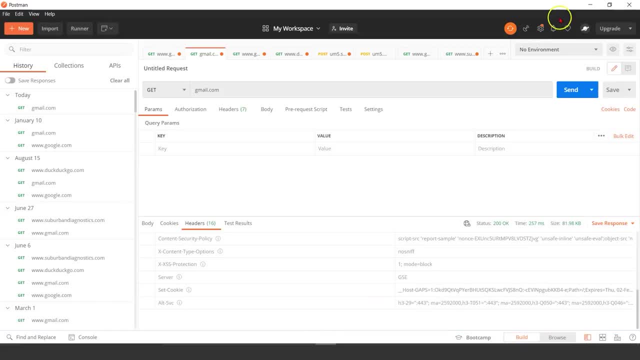 to the website and then this is the email address. So this is the address, right? They have added few, but this is the address code for the website, So I can just keep on going for minutes, right? and then when I send it, it's going to take a while for the manner. 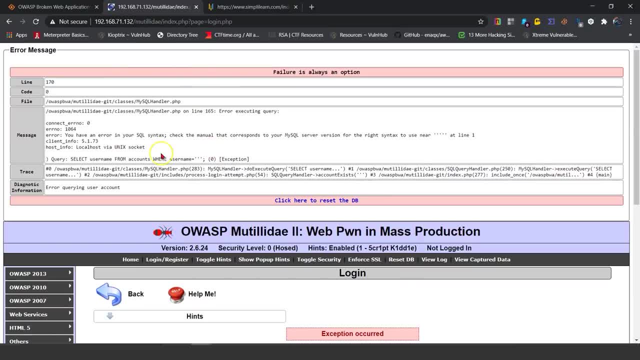 of sending those letters. So again, the earlier you send these letters, then your adress will start sending letters. That would be a lot right. So we don't want that. So that's just some examples. So if right, you can see that the application converted this into a sequel query. so 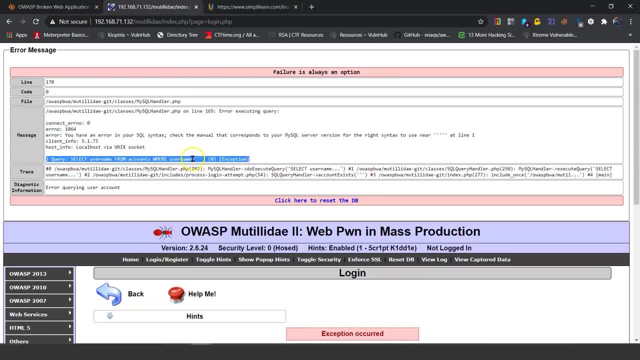 the query was select username from accounts where the username in quotes single quotes and we use this quote right, the single quote right there. so that's where we use that operator and that's where the exception error occurred. so these are the kind of queries that are structured by the application and 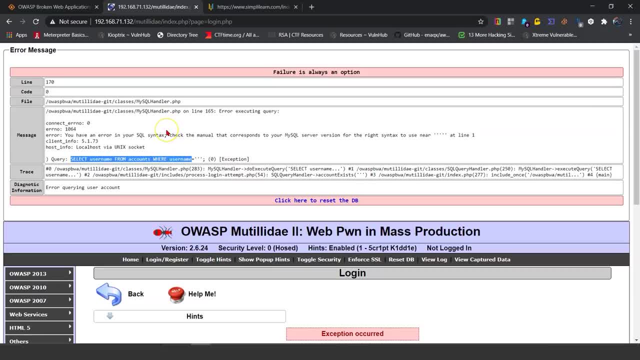 then taken on to the database for execution. when we type in it is a HTTP GET request with the username and password within that query that is sent to the application. the application converts it into a sequel query, sends it to the database and the database responds with the appropriate response. 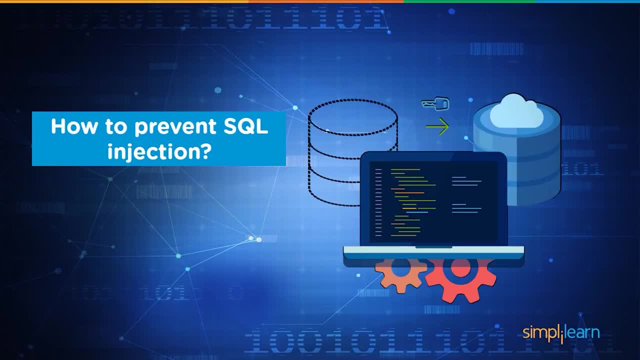 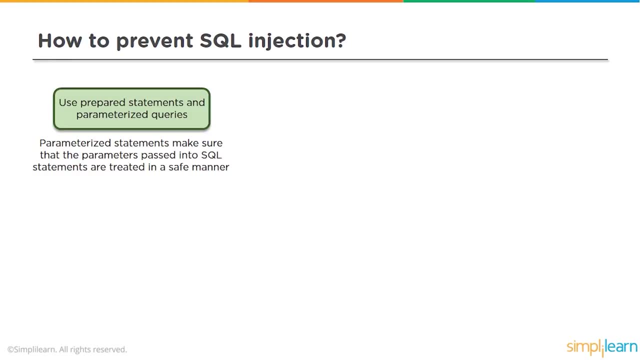 so how do we prevent SQL injection in the first place? use prepared statement and parameterized queries. these statements make sure that the parameters passed into SQL statements are treated in the same way as the parameters passed into SQL statements are treated in the safe manner. so, for example, we saw that the single code was an operator. this: 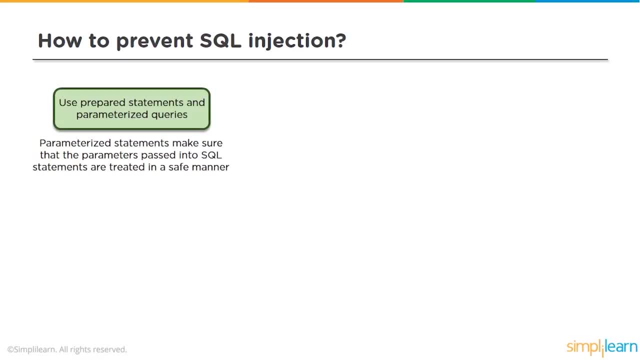 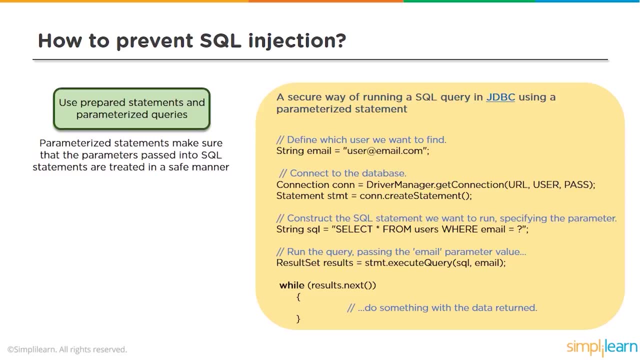 shouldn't be allowed to be utilized in the first place. right, so here? what we are doing here is a secure way of running a sequel query in the JDBC using a parameterized statement. define which user we want to find. so there's a string. the email comes in connection to the database. we are going to figure out how. 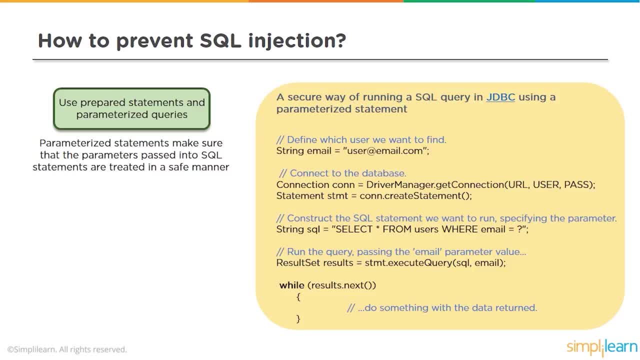 the connection is going to be passed, how it is going to be created. construct the sequel statement. we want to run specifying the parameter, right? so we define: how is it going to be created, what is going to be created, what can be passed to the database and what should not be passed to the database. so that is. 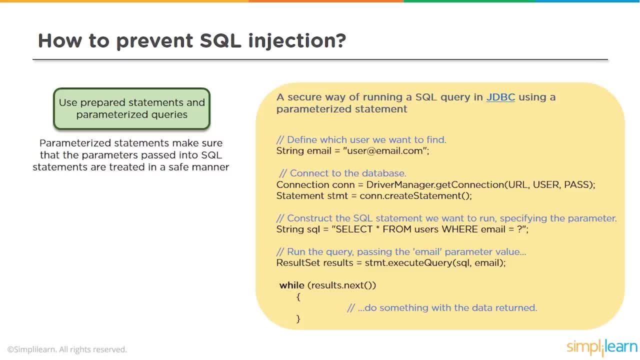 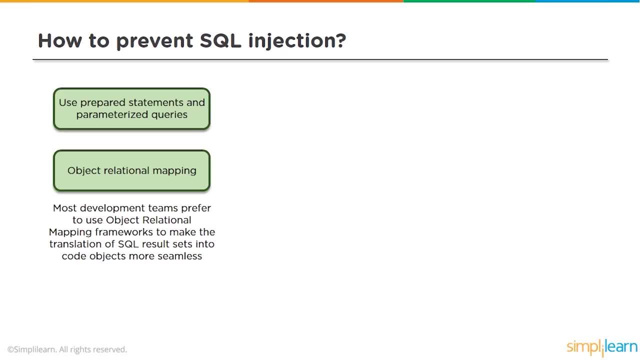 one way of utilizing prepared statements and parameterized queries. then we have object relational mapping. most development teams prefer to use object relational mapping frameworks to evade the translation of sequel results set into code objects more seamlessly. so this is an example of object relational mapping where we map certain 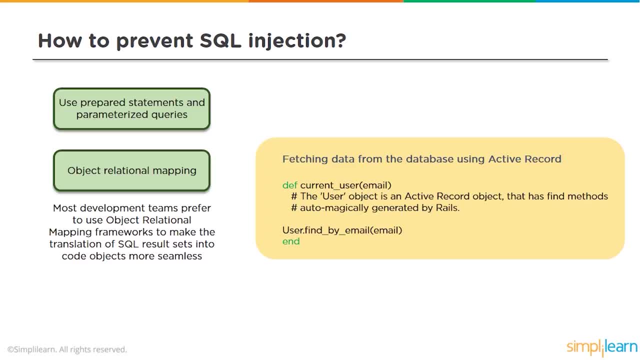 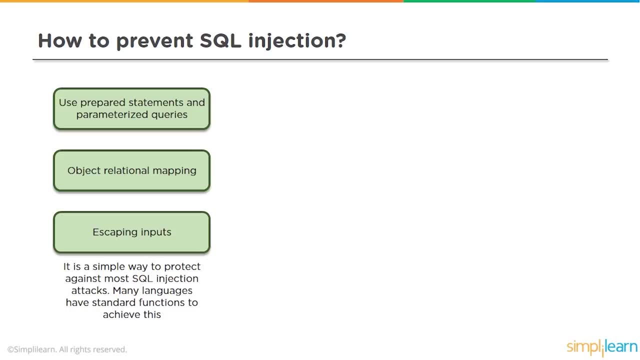 objects and allow that to be executed, and then escaping inputs in a simple way to protect against most sequel injection attacks. many languages have standard functions to achieve this right, so you need to be very careful while using escape characters in your code base when a sequel statement is constructed, not 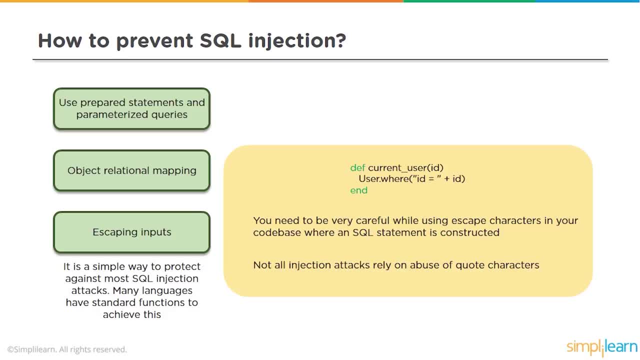 all injection attacks rely on abuse of code characters. so you need to know what characters are being utilized in the configuration that you have created. in the structure that you have created, in the code that you have created, which characters are being recognized as operators. you need to sanitize those. 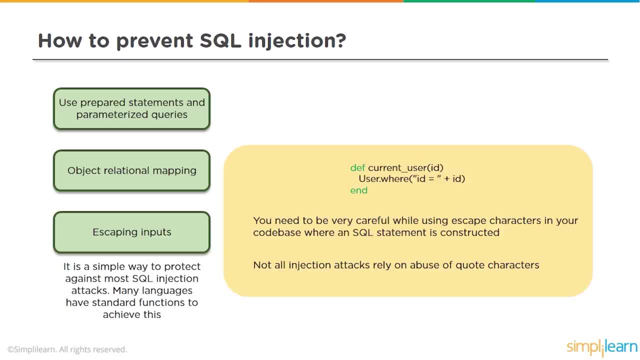 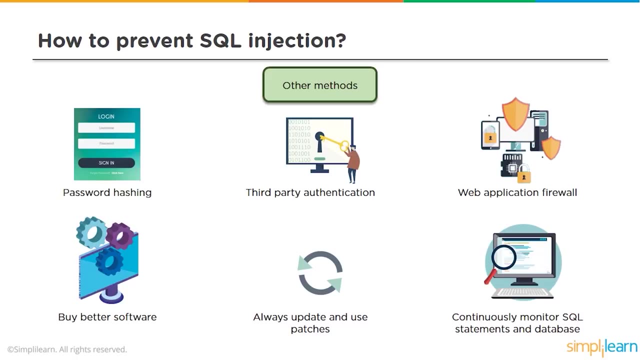 operators and you need to basically ensure that these operators cannot be accepted as user input. if they are, there be layout by the application and they never reached the database. other methods of preventing sequel injection: our password hashing so that you can configure SQL to rationalize on the. 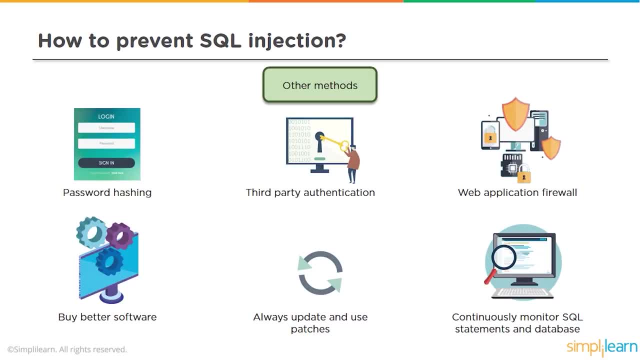 thực Им, So that passwords cannot be bypassed, the passwords cannot be recovered, passwords cannot be cracked. Third-party authentication: you use OAuth or some other service for a single sign-on mechanism. Thus you rely on a third party to maintain the security of authentication, and what kind of parameters are passed. 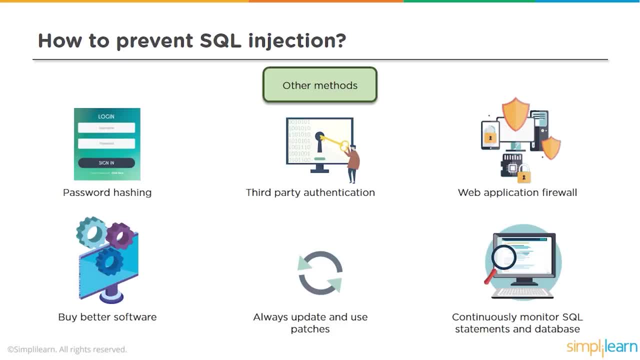 For example, using LinkedIn logins or Facebook logins. right For the layman. you normally go on to Facebook and you allow if you're using a game. right, If you start playing a game, you're allowed to log into the game using your Facebook credentials or your Google credentials. 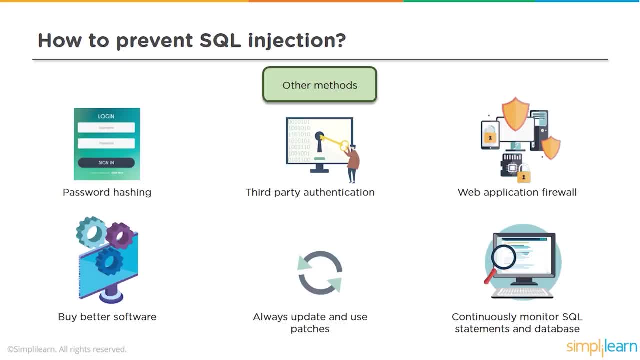 Now, that is not just for ease of use, but the game user, the developer, has outsourced the authentication mechanisms to third parties such as Facebook or Google, because they understand that that authentication mechanism is as safe as can be. Facebook and Google are wealthy organizations, hire a lot of security experts, and the development for their authentication mechanisms is top-notch. 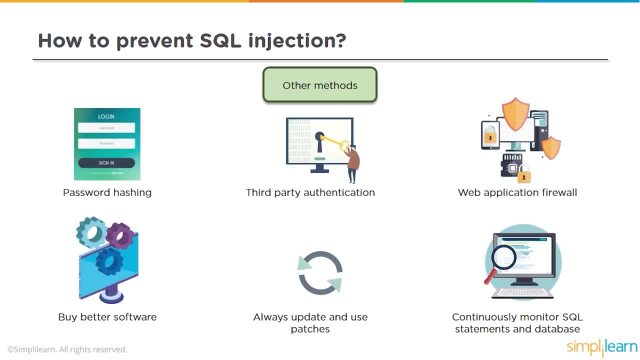 A small organization cannot spend that kind of money on security itself, right? So you use a third-party authentication mechanism to ensure that these kind of attacks may not happen. Then web application firewalls: Having a web application firewall and configuring it properly for SQL injection attacks is one of the sure-shot methods of authentication. 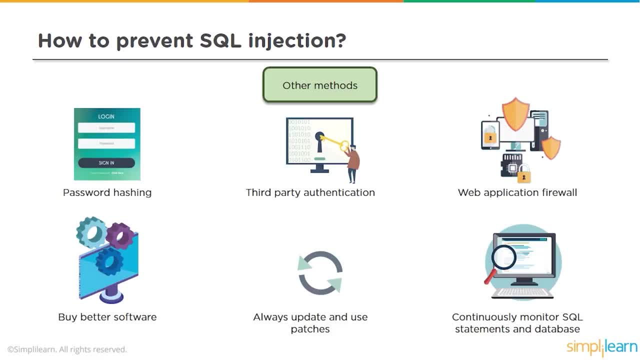 The web application firewall is a good example of how you can stop the application from mitigating or minimizing the threat in the first place. So at this point in time, you have realized that the application has some vulnerabilities for SQL injection And instead of recoding or restructuring the application, you want to take the easier way out or the cheaper way out. 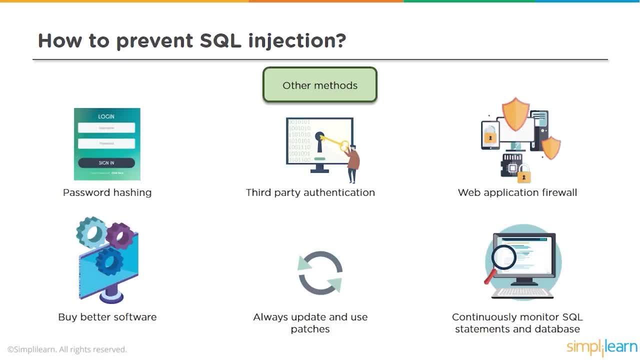 So what you do is you install a web application firewall and you configure the web application firewall to identify malicious queries and stop them at the firewall level itself, So they never reach the application And thus the vulnerabilities on the application don't get executed. 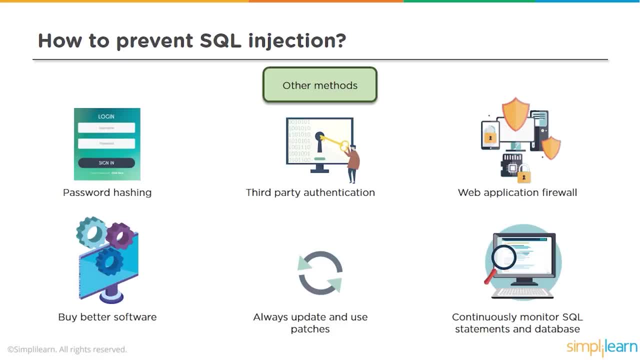 Buy better software and keep on updating the software. So it's not necessary that once you have a software, you install it. it's going to be safe for life. New vulnerabilities are discovered every day, every hour, And it may so happen. what is secure today may be completely insecure tomorrow or the day after right.